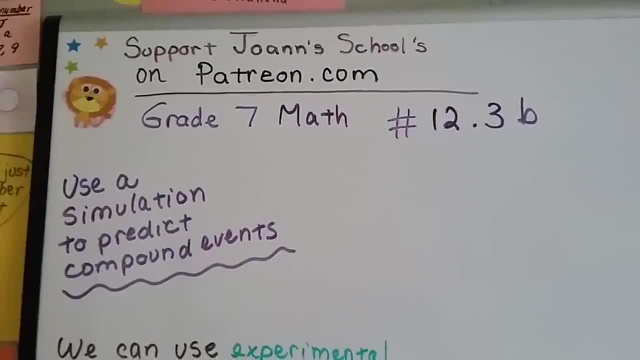 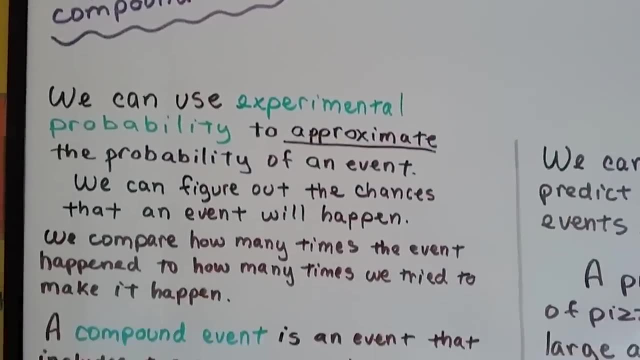 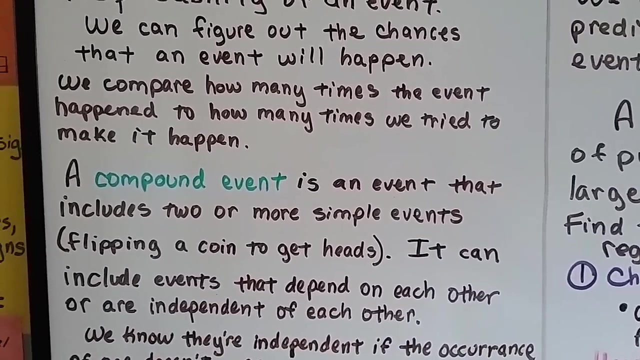 Grade 7, math number 12.3b uses simulation to predict compound events. We can use experimental probability to approximate the probability of an event. We can figure out the chances of an event will happen. We compare how many times the event happened to how many times we tried to make. 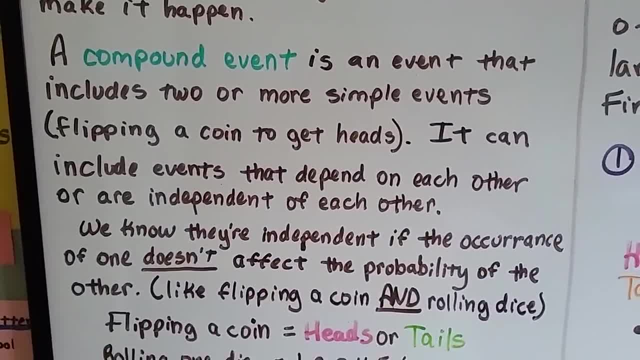 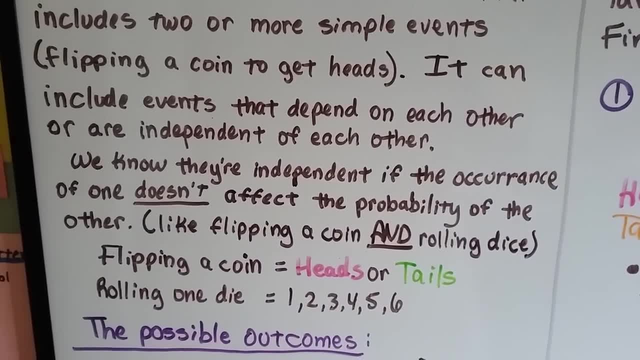 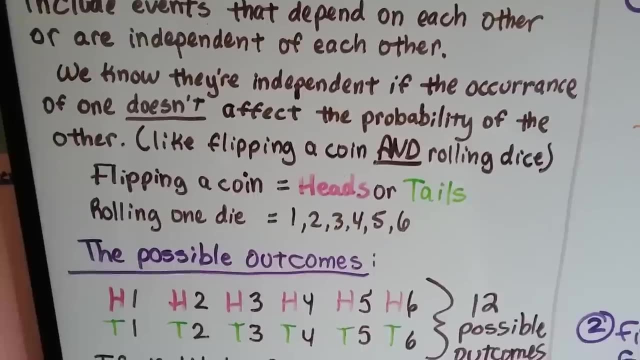 it happen. A compound event is an event that includes two or more simple events, like flipping a coin to get heads, and it can include events that depend on each other or are independent of each other. We know they're independent if the occurrence of one doesn't affect the probability. 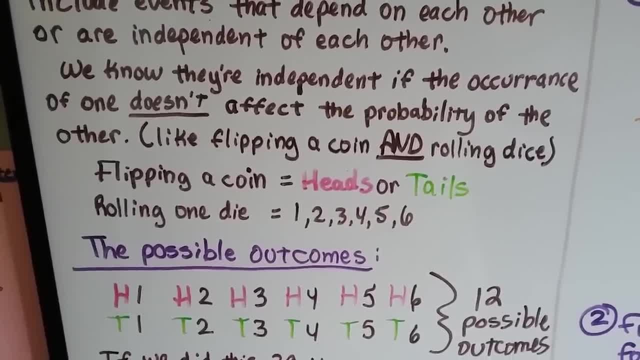 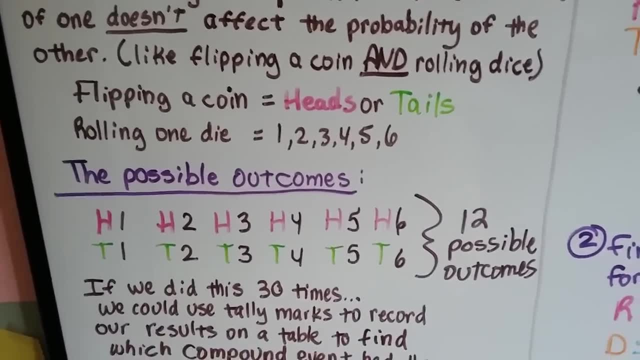 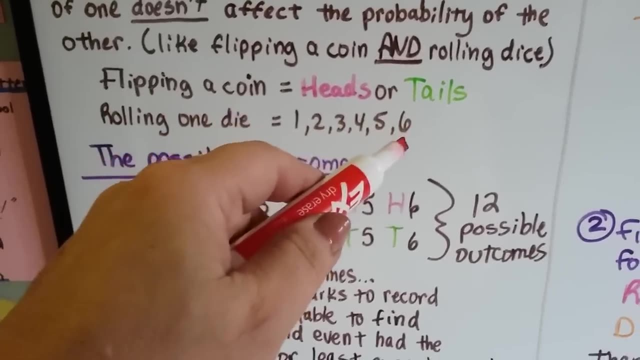 of the other, like flipping a coin and rolling dice. Flipping a coin doesn't affect what happens when we roll the dice, does it? So flipping a coin would be getting heads or tails, and rolling one die would be one, two, three, five or one, two, three, four, five or six. 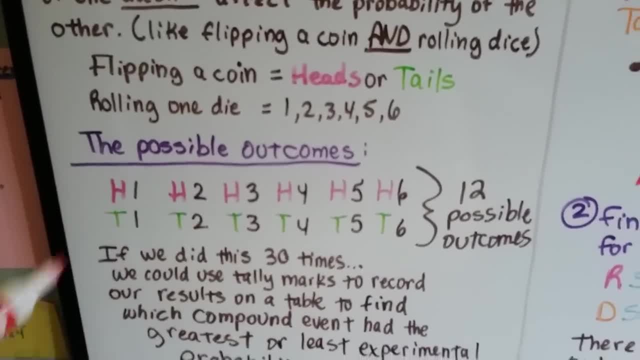 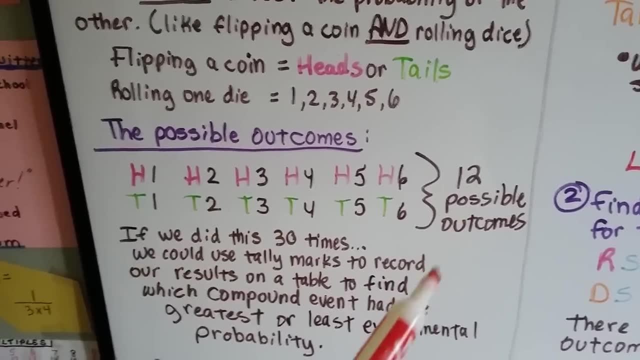 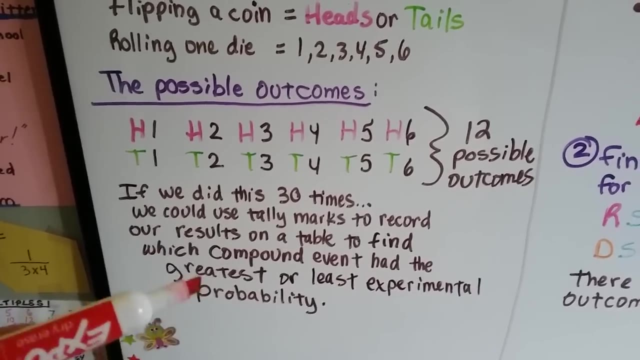 Right, Because that would be on one die. So the possible outcomes would be heads or tails of one, two, three, four, five or six. That's six possible outcomes for each. That's a total of twelve outcomes, And if we did this 30 times we could make tally marks on a table and record our results. 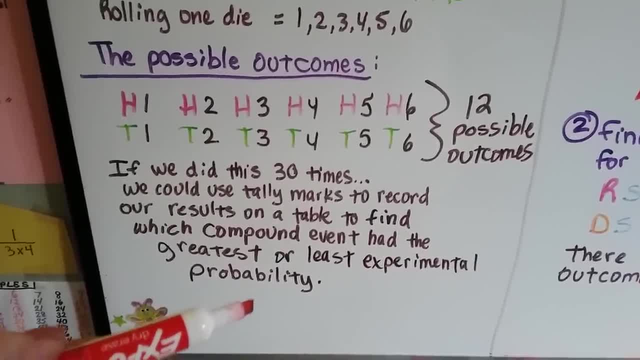 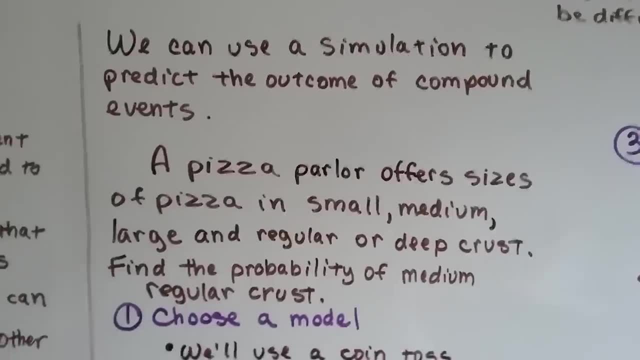 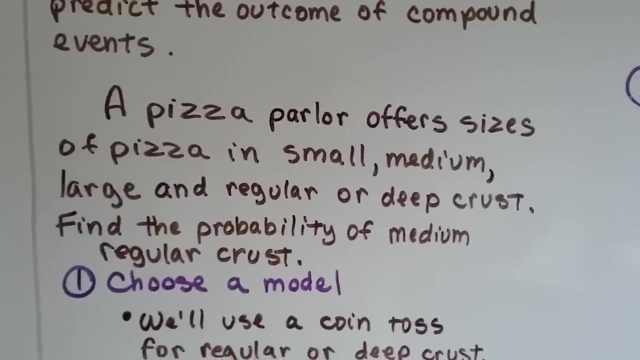 Right. Then we could find out which compound event had the greatest or least experimental probability. So we can also use a simulation to predict the outcome of an event. So let's say a pizza parlor offers sizes of pizza in small, medium, large and there's a regular or deep crust. 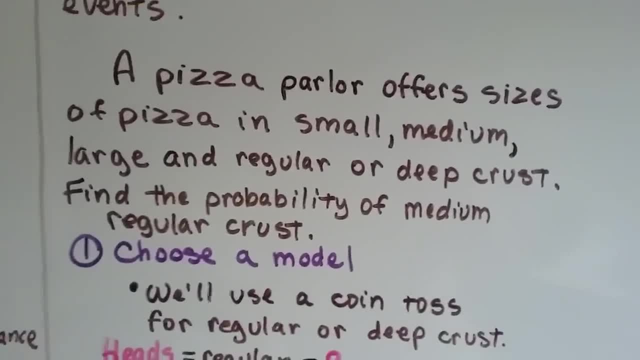 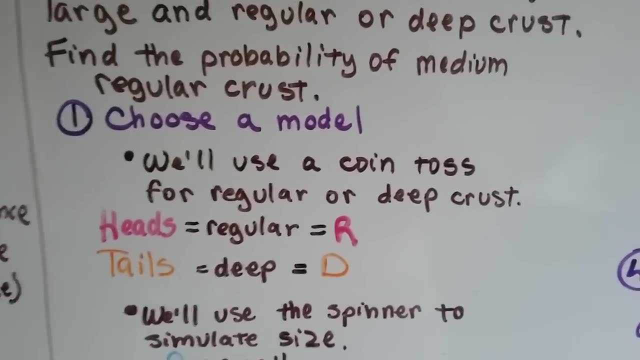 So you have a regular crust or a deep crust, So we're going to find the probability of a medium regular crust pizza. So we choose a model. So we're going to use a coin toss for the regular or deep crust and heads is going to be regular. 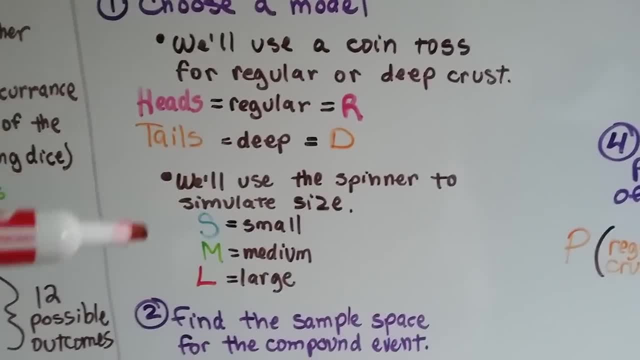 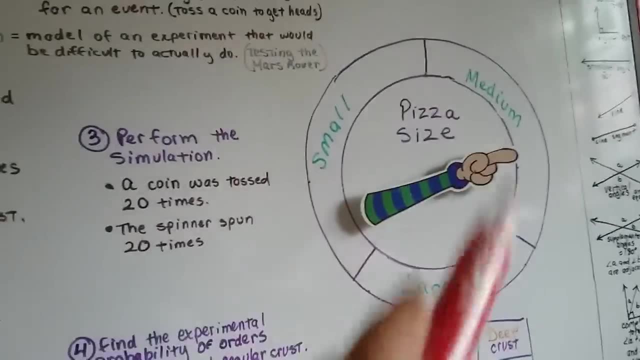 and tails is going to be the deep crust And we'll use our spinner to simulate small, medium or large. So I've got it split into small, medium and large so that it can be spun to see where it's going to land. 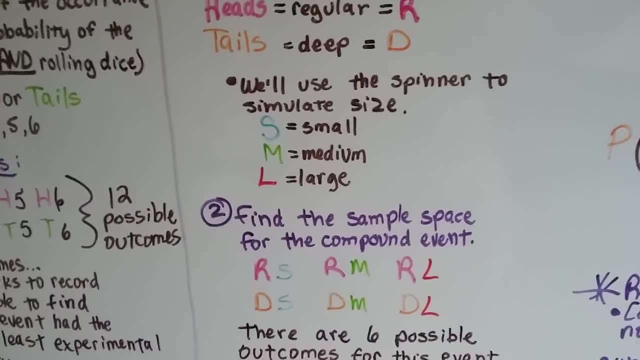 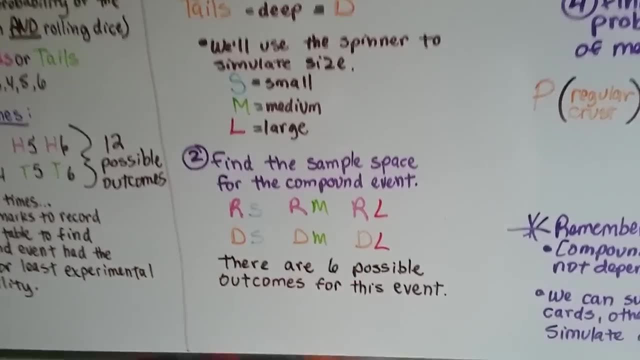 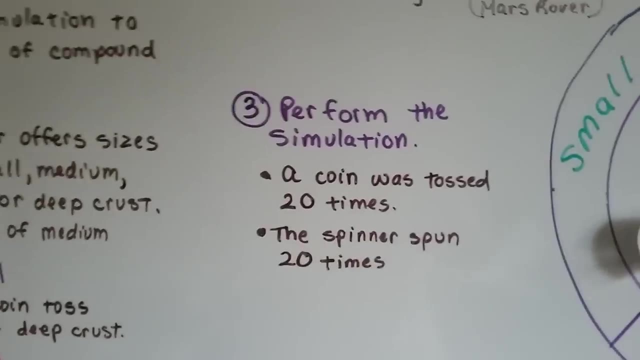 Okay, We find the sample space for the compound event. So regular, small, regular, medium, regular, large, deep dish. small deep dish, medium deep, dish, large. So there's six possible outcomes for this event, Aren't there Alright? So now the next thing we do is perform the simulation. So a coin was tossed 20 times and I spun the spinner 20 times. 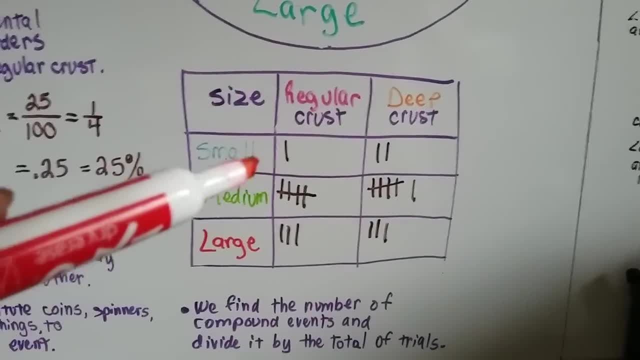 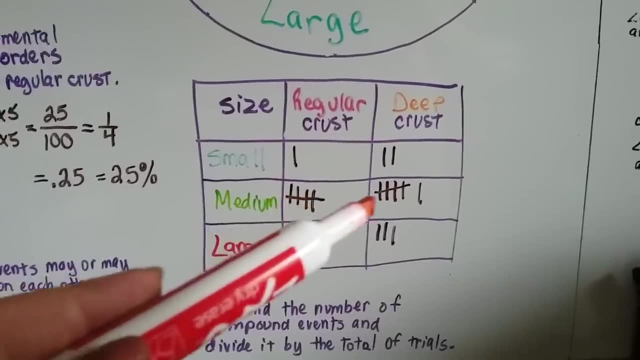 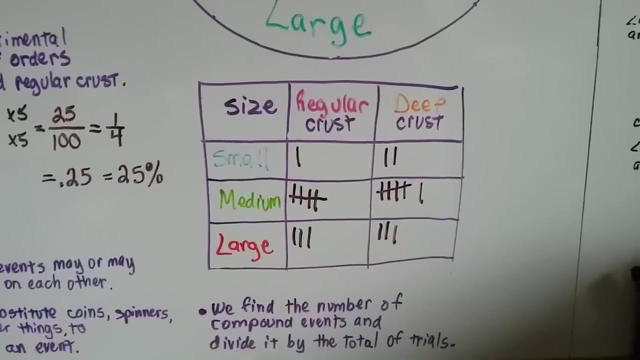 And this is what happened. I got one small regular crust. two times it landed on deep crust small, five on the regular medium, six on the deep crust medium, three on the regular large and three on the deep crust large. So we were looking for regular crust medium. It landed on it five times out of 20.. 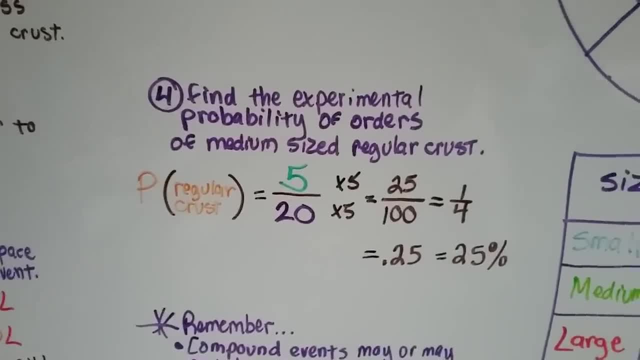 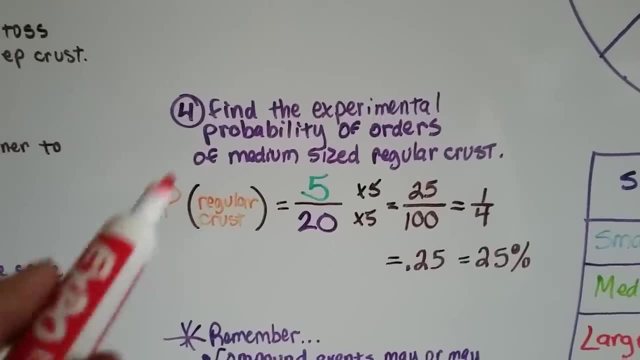 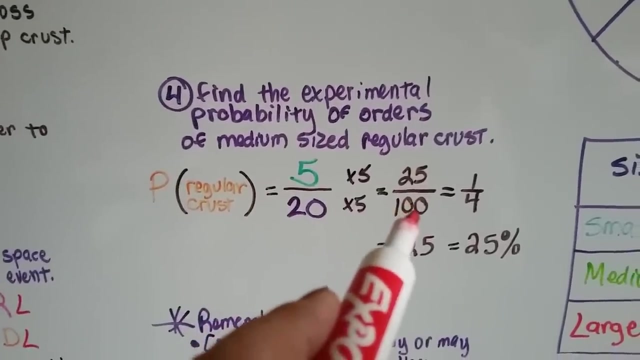 So the next step of find the experimental probability of orders of medium sized regular crust, the probability of regular crust, that's what this means. P regular crust is the probability of regular crust equals five out of 20.. What does 20 need to become 100?? Well, it needs to be multiplied by five. 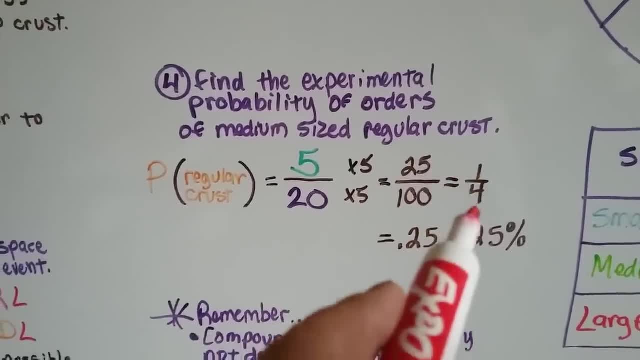 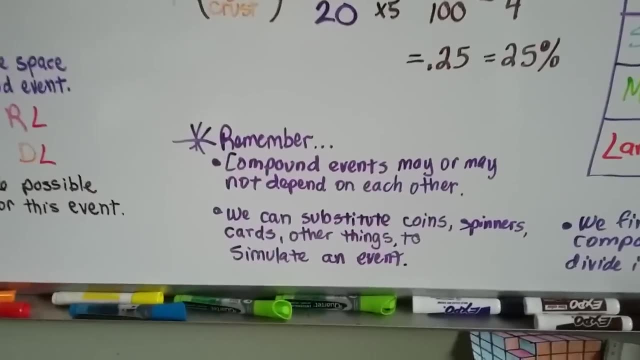 So we multiply both by five, We get 25 over 100.. That's one fourth or 0.25 or 25%, Right? So we've got to remember that compound events may or may not depend on each other. They may not. 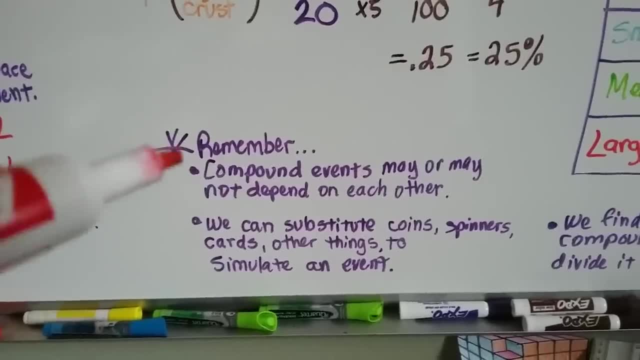 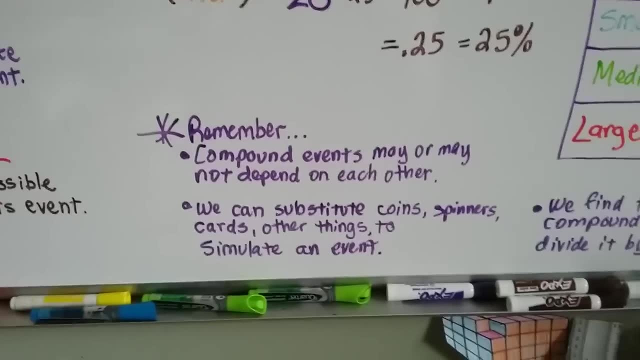 They may be independent or they may depend on each other, So don't think they always have to be independent. Okay, And we can substitute coins and spinners and playing cards and other things to simulate an event. So we need to find the number of compound events and divide it by the total of the trials. Okay, 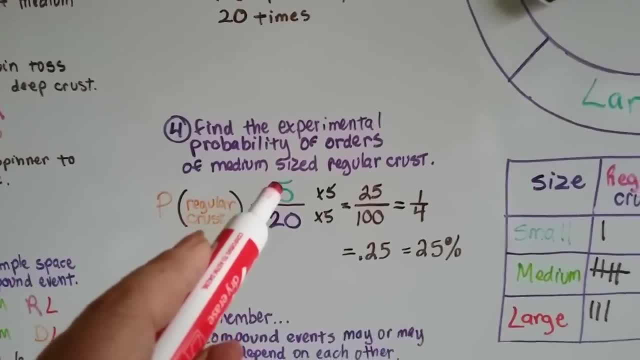 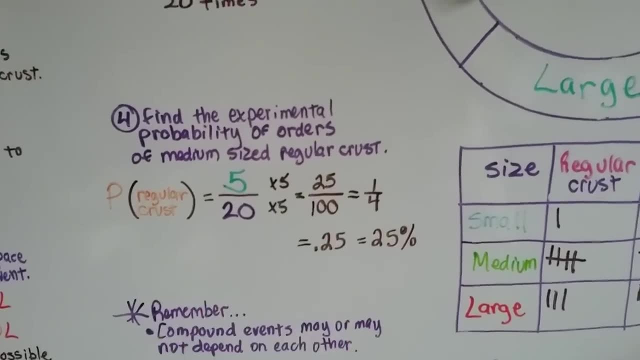 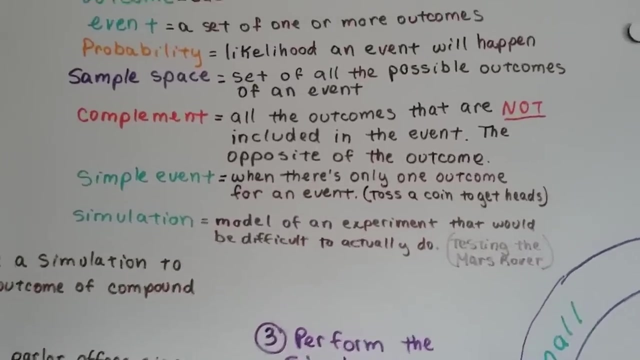 So we find the number of the compound events, See, And we divide it by the number of trials, and then we get the percentage of the decimal or the fraction. Okay, So just remember, a simulation is a model of an experiment that would be too difficult to actually do. 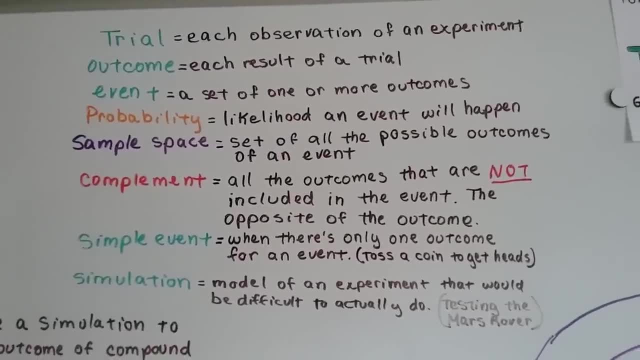 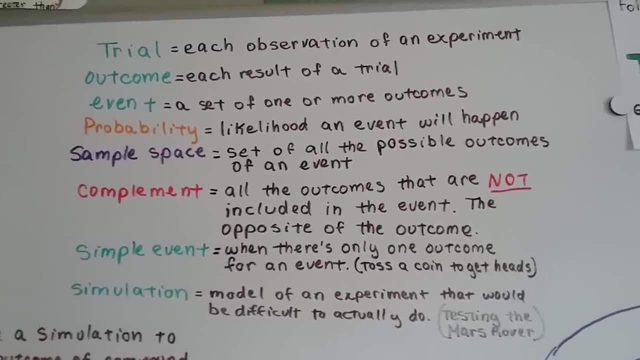 Here's all of our definitions. I'm going to go over them again in the beginning of our next video, And it would be like them testing the Mars Rover in their laboratory, because they can't test and build it on Mars, They can't get a hundred engineers and all the people that worked on it to Mars to work on it. 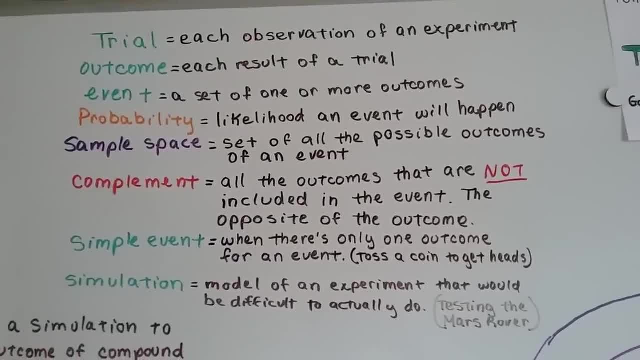 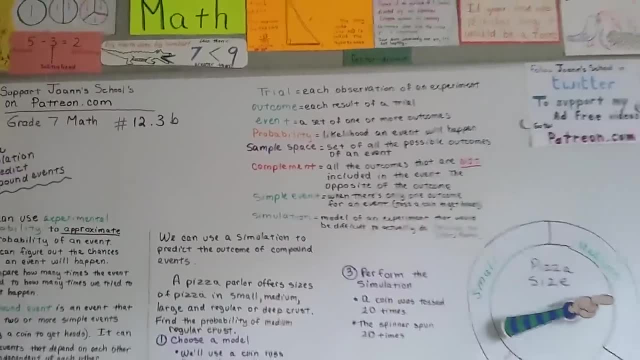 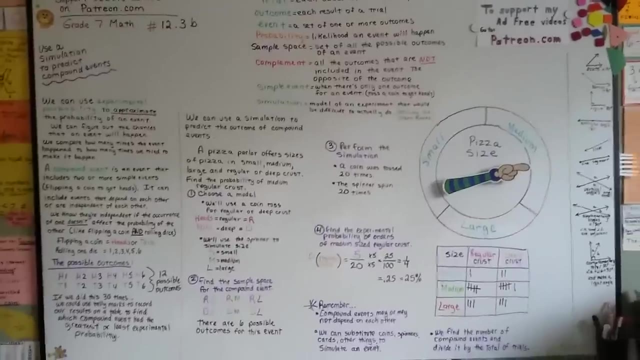 So they had to simulate it in the lab and how its wheels would turn over the rocks and everything on Mars. Okay, All right. So our next video. we're going to talk about experimental probability and making qualitative predictions. There's qualitative and quantitative. 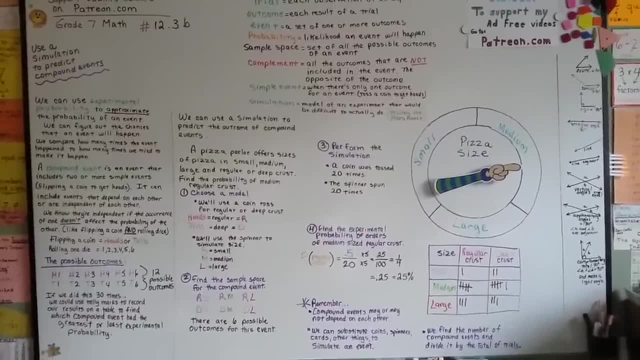 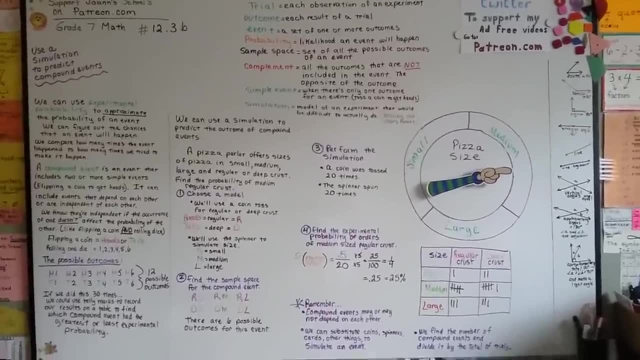 And in our next video we're going to talk about the qualitative predictions. Okay, I really hope you're doing well. I'm voting for you here. I'm really rooting for you, Okay, So keep trying And we're going to get through this. 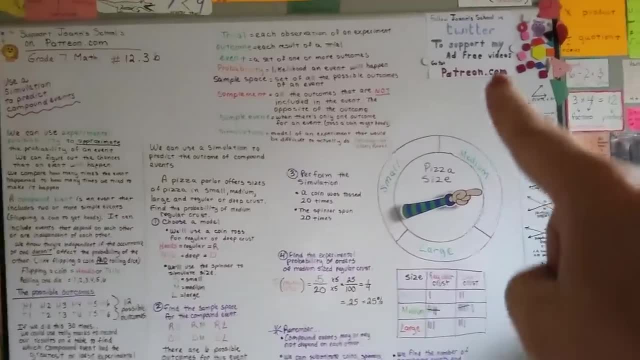 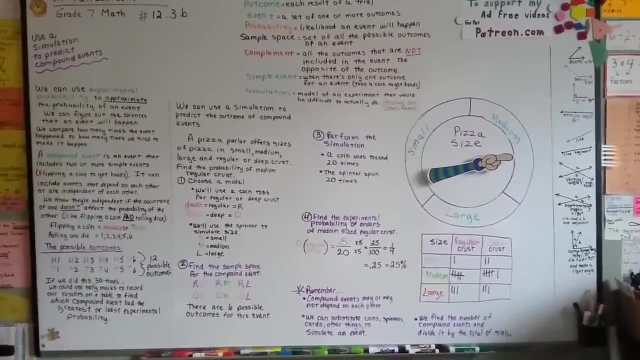 We're almost done with seventh grade math. And don't forget- don't forget that I'm on Twitter And if you want a copy of a picture of any of these as a study guide, just let me know. Send me a message on Twitter and I'll post it. 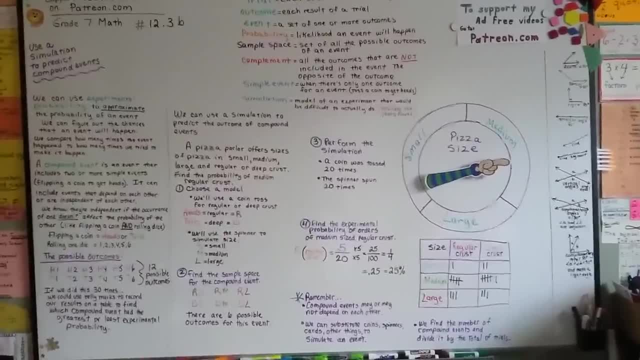 All right, And don't forget to hit the like button. It's the only way I know if I'm helping anybody. Okay, See you next video. Bye. 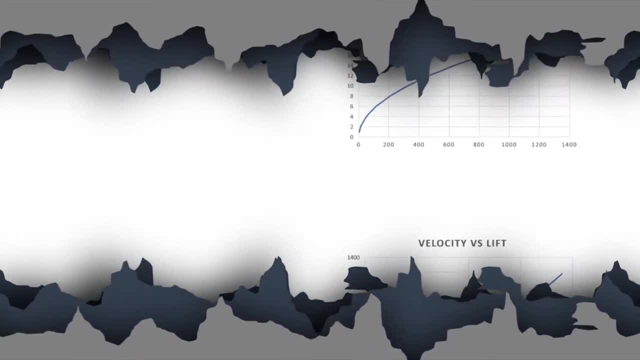 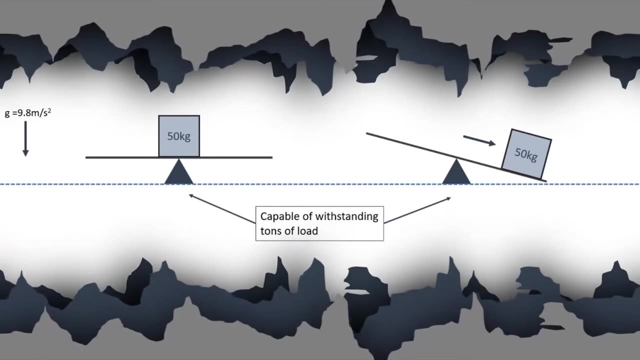 Welcome to aerodynamics in minutes. Today we are going to understand what is movement, what is center of pressure and what is an aerodynamic center. In the two diagrams, the pivot base is a spin joint, As you can see, placing 50 kg perfectly. 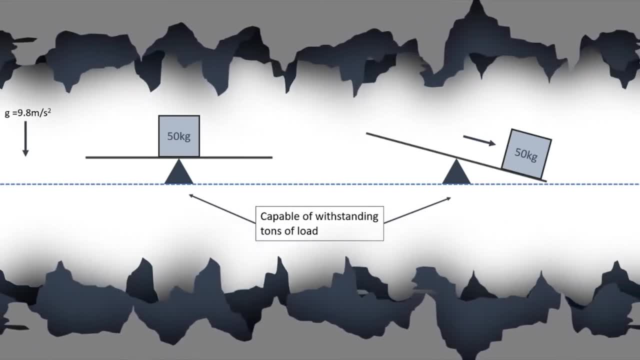 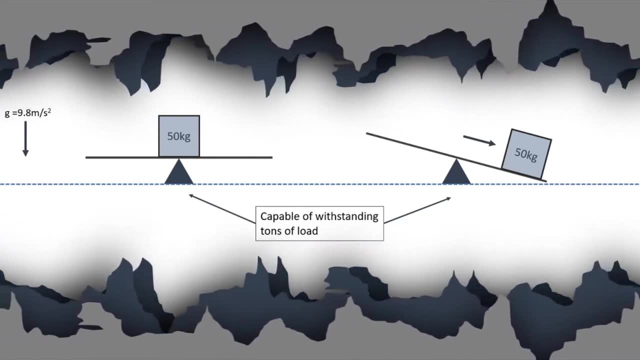 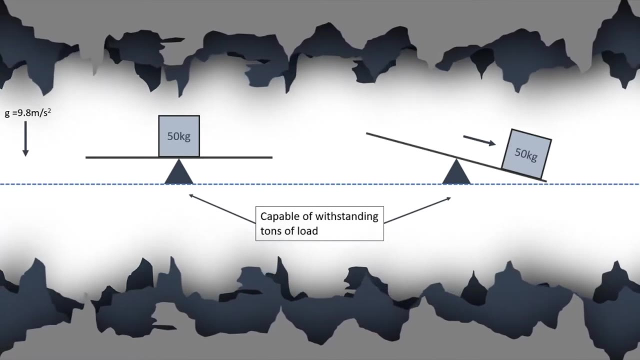 centered in the pivot base, the seesaw is balanced, But moving it from the middle makes the seesaw unbalanced. This unbalance is created due to the movement generated by the weight we have placed. The magnitude of the movement increases as the distance increases. We can find the moment. 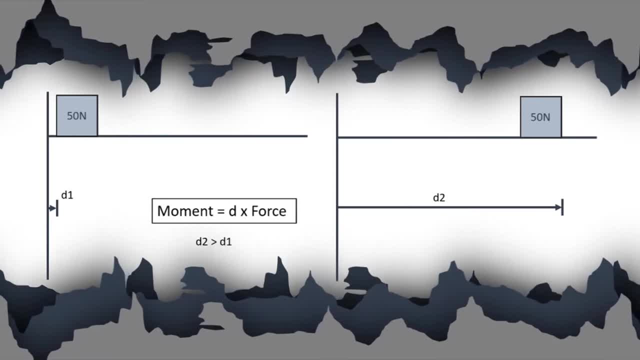 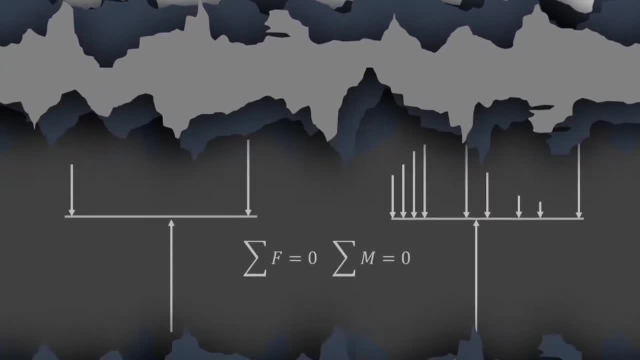 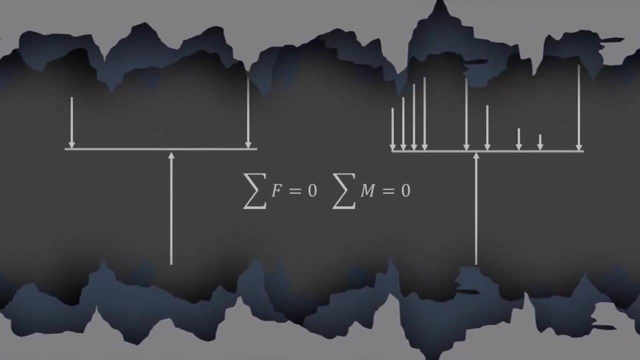 generated using the formula Force into Distance. I think you don't need any explanations for this formula. as you can easily understand, There may be N number of forces with different magnitudes acting on the body. All these forces acting on the body can be replaced by a single resultant force. 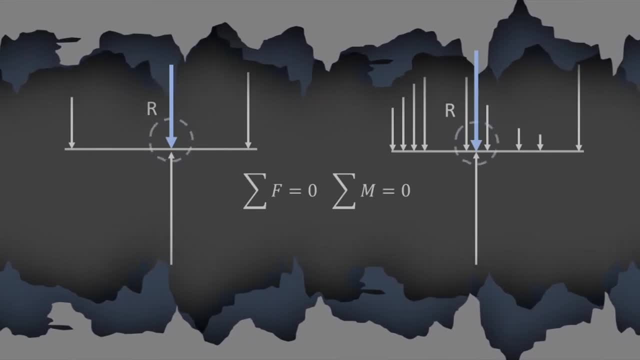 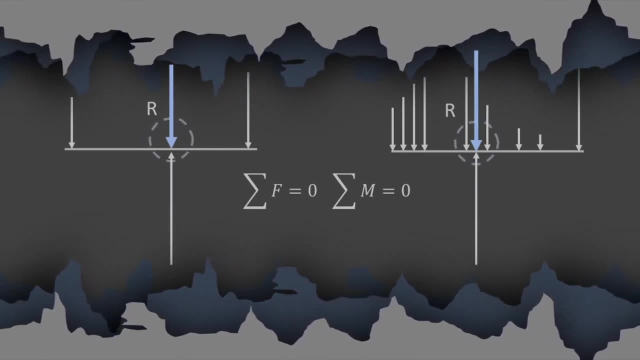 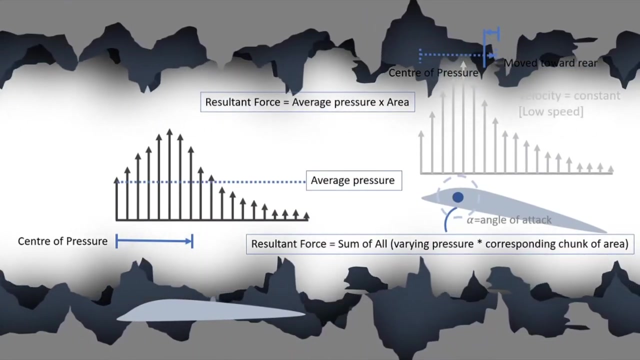 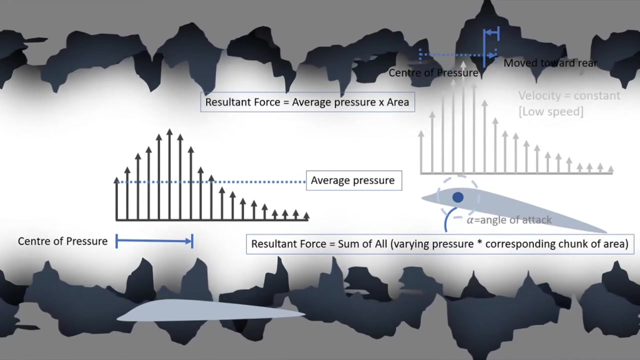 and the magnitude and the position this force are found using the body at equilibrium condition, that is, sum of all forces and the sum of all moments is zero. these arrows are the lift distribution over the top surface of the airfoil to locate the center of pressure. think all the varying pressure at each chunk of area as a force. the magnitude: